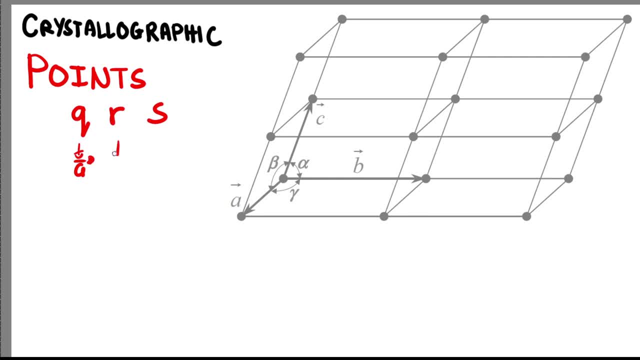 So for Q it's along A, For R it's along the B direction And for S it's along the C direction. So, for example, let's take this origin, So in our origin, since it's an origin, we didn't translate along QRS or along A, B, C. 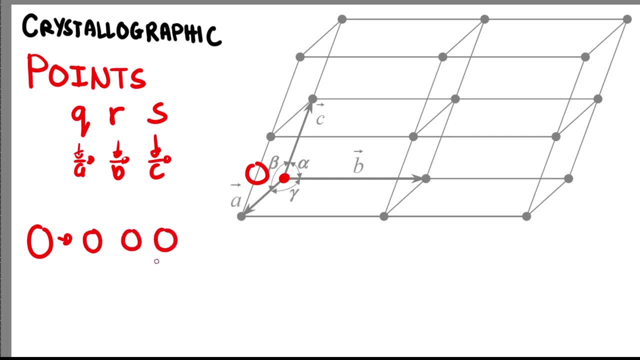 So QRS would be 0, 0, 0.. So when we're writing crystallographic points, we'll see here that we don't put commas, We don't put parentheses or brackets or anything, We just put the numbers 0, 0, 0. 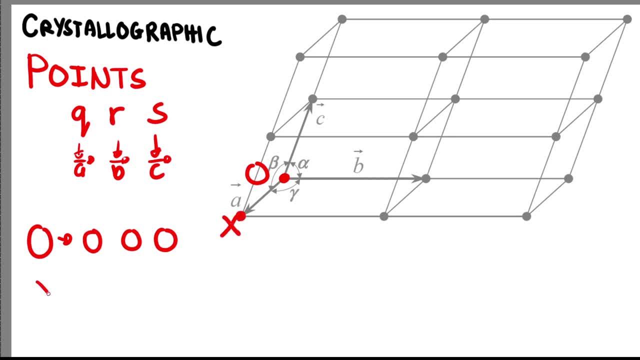 How about this one? Let's say, this is point X. For point X, this would be one unit along A, no units along B and C. So this would be 1, 0, 0.. Now let's take, for example, this point here: 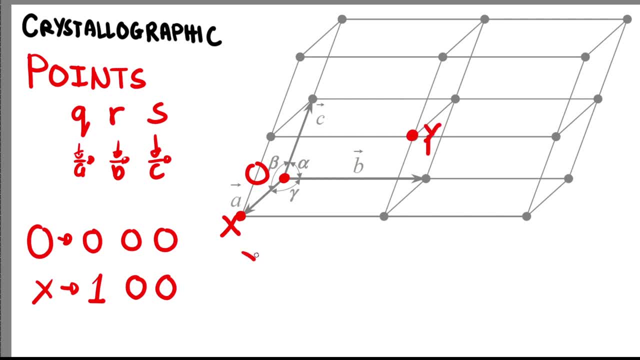 Let's call this point Y. For point Y, we're translating: one unit along A here, one unit along B here and one unit along C to get to this point. So this will be 1,, 1,, 1.. 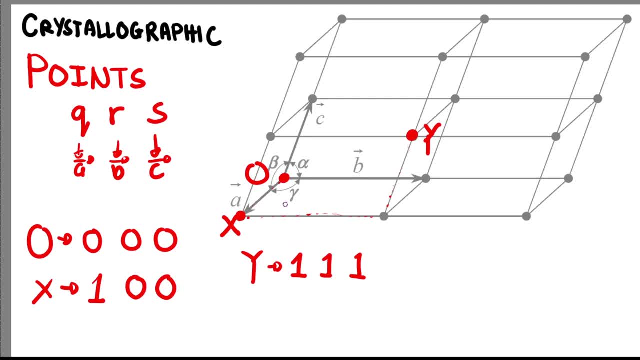 So notice here that even though the lengths are different, or A, B and C, they're still 1, 1, 1.. Since recall that we're basing off these vectors and QRS are fractional distances along A, B and C directions. 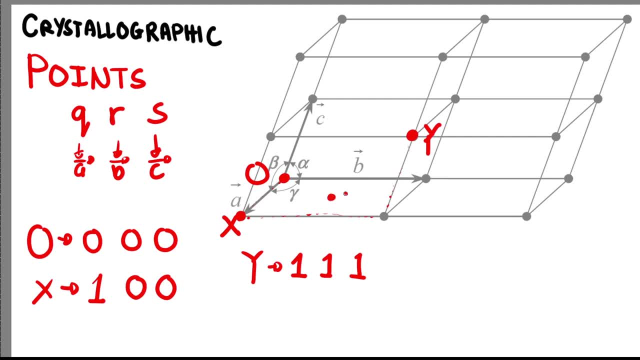 We can also have fractions. So for example, we have a point here, Point C. So for point C, let's say this is one-half along A and one-half along B. Point Z will then be one-half one-half and your S-NATAN will be 0.. 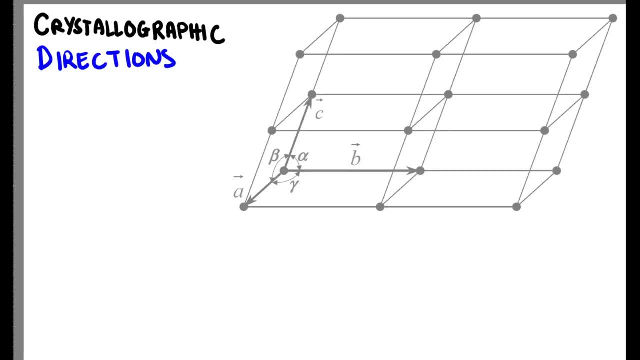 So now we go into our crystallographic direction. So this is defined as a line directed between two crystallographic points. So this will become a vector. So denotations for our crystallographic direction something like this: have u, v- w, where u, v and w. 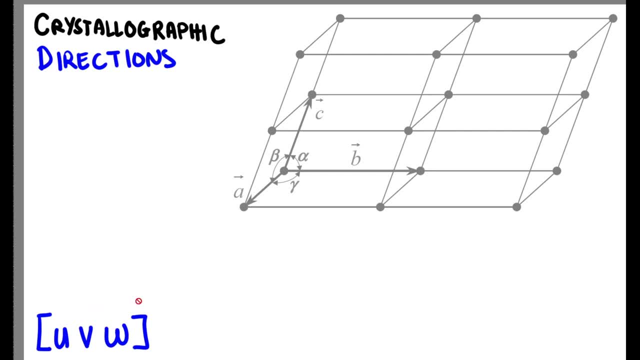 corresponds in the directions along a, b and c respectively, And this is enclosed in our square brackets here without any commas. So to obtain our crystallographic directions, what I personally do is: first I find the coordinates of the head and tail of our direction vector. 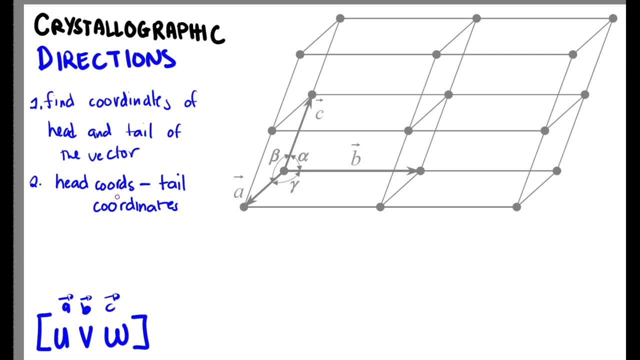 Then I subtract the tail coordinates from the head coordinates for each of u, v and w, corresponding to the points x, q, r, s for each of the tail and the head. And then, lastly, if needed, I subtract the tail coordinates from the head coordinates for each of u, v and w. 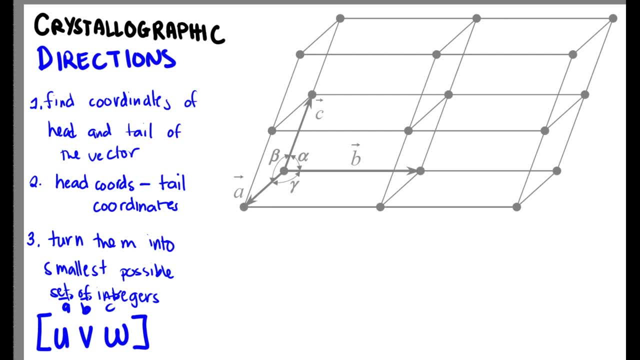 and I turn them into the smallest possible set of integers that I can And I enclose this again in our square brackets. So now let's go for an example. Let's say we have this direction here in our unit cell. Let's call this direction, direction m, So to get the index of this. 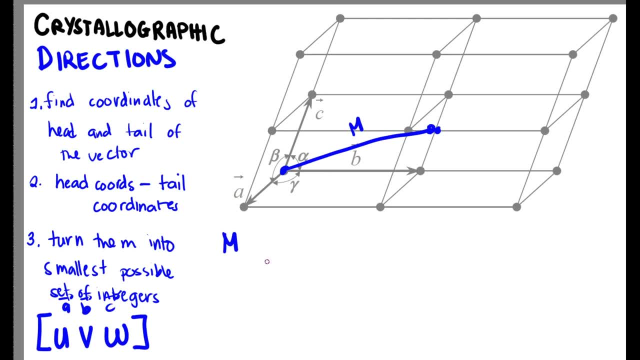 direction. we use the following steps here. So for m, the tail is here and its head is here, And then the coordinates of our head is along b and along c. Along b, it's 1.. Along a, 0.. 0,, 1, and along c it's 1. half Meanwhile for its tail. 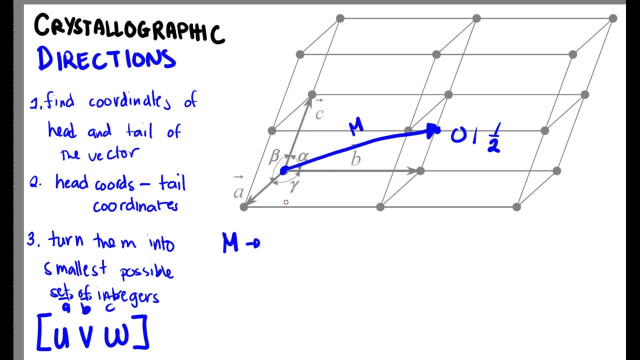 conveniently, I put it in the origin so that we can see This will become 0, 0, 0.. So to get the direction, head coordinates minus tail coordinates. So we have: for u it's equal to 0, minus 0.. For v equal to 1, minus 0. And for c or for w, sorry. 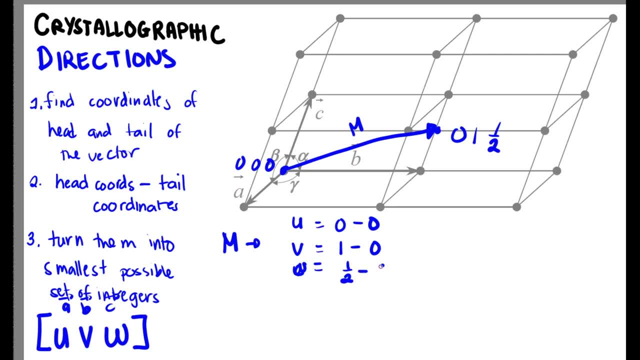 it will become 1 half minus 0.. u v w will be equal to 0, 1, 1. 1 half u v w equal to 0, 1, 1 half, But since we have a fraction here, 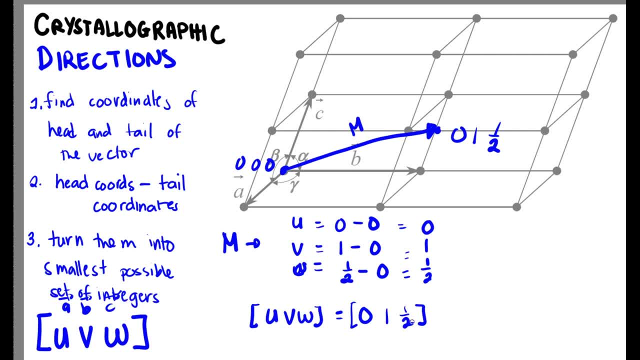 we need to turn them to the smallest possible set of integers here. So we do that by multiplying each of these by 2.. And the correct direction would be 0,, 2,, 1.. And close in brackets. And now let's try a different example. Let's use this direction here: Going dito, So it's along. 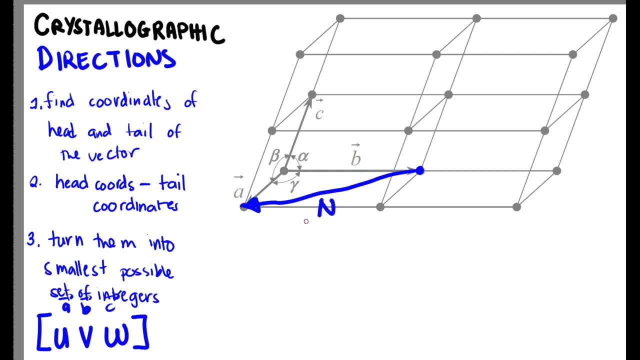 the basal plane a, b, Let's call this vector n. So vector n, yung head nya, is at this point, and this point is 1, 0, 0.. Yung vector, yung tail naman ng vector natin, it's at this point. 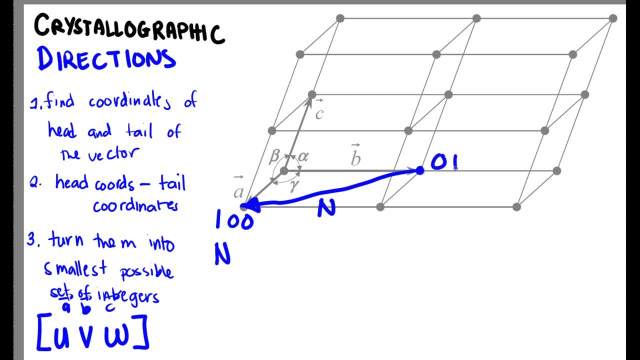 which we know as 0, 1, 0. So to get yung u v w natin dito, makita natin we have: u is head minus tail, So we have 1, minus 0. Yung second naman natin for v, 0, minus 1.. And for c: 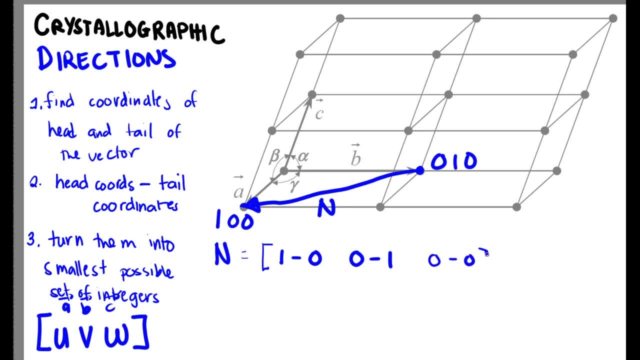 we would have 0, minus 0. So this will become 1, minus 0 is 1. 0, minus 1, negative: 1. 0, minus 0, 0.. So for our index notation, for our Miller index notation, yung n natin pag meron tayong negative. 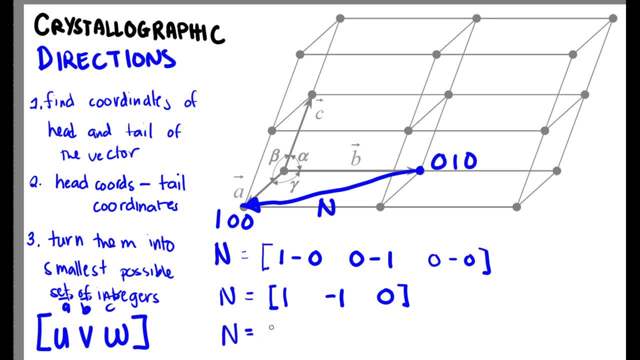 na value. para hindi tayong malito, ang ginagawa natin is sinalagayin natin yung bar sa taas, So yung negative, parang inaakit lang natin magiging 1 bar 0 sya. 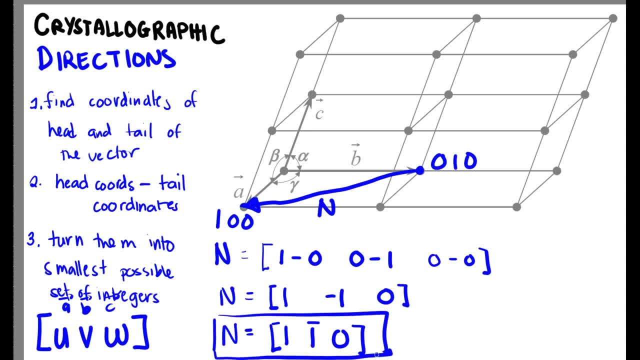 So this would be our direction for the vector shown here. So one final example for our crystallographic direction. let's say naman, we want to visualize what the direction would look like in our crystal. So let's say we're given this direction. 1,, 2,, 2 direction. 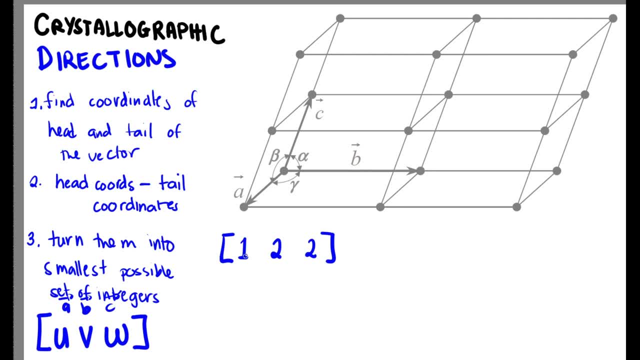 So in this case, we just reverse what we did before, So 1,, 2,, 2.. Ang mangyari dyan. We can take this As the coordinates of the head, And let's just put the direction or the tail of the vector at 0, 0, 0.. 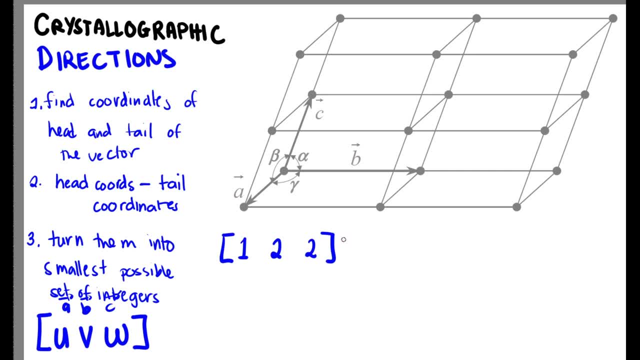 So it's just as if we are looking for the points 1, 2, 2 here. So you have 1, 1, 2, 1, 2.. This will be your tail. This will be your head. 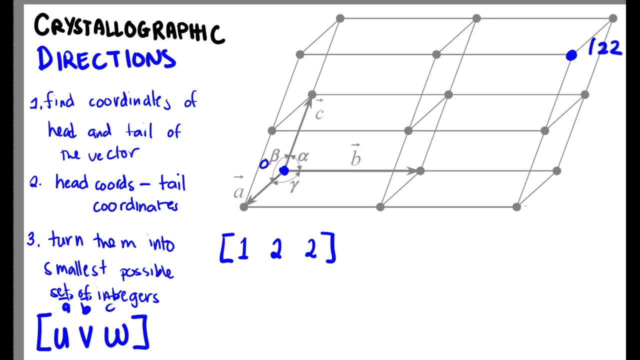 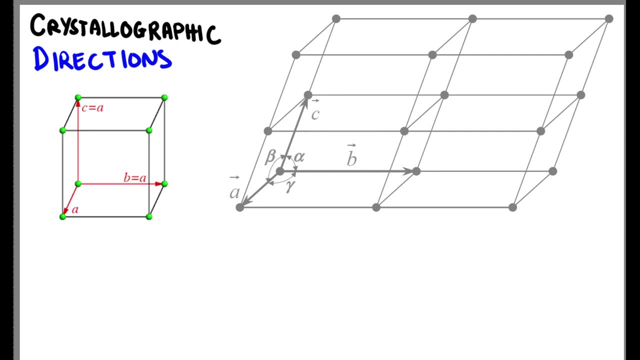 1, 2, 2.. This is 0, 0, 0.. And your direction would be eto. This is 0, 0, 0.. And the direction would be eto. For some crystal structures, several non-parallel directions with different indices could be. 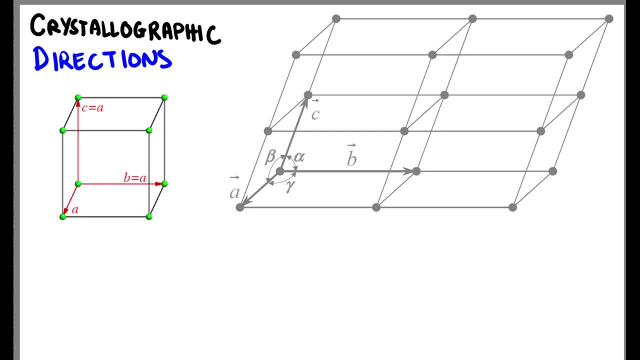 crystallographically equivalent, Meaning that the spacing of atoms along each direction might be the same. So in that case we might group these directions together in what we call a family of directions. So pag meron tayong family of directions ang, meron tayong family of directions ang, 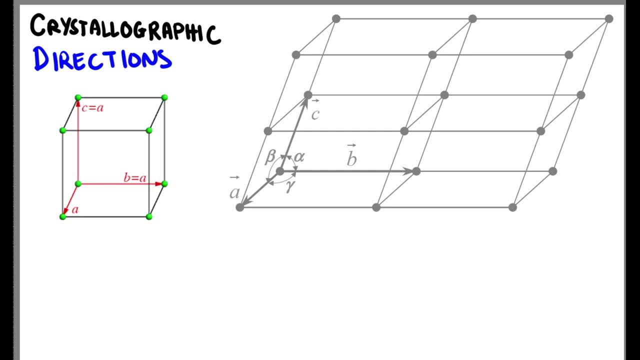 notation natin for that one is this one. so we have yung less than sign and we have yung index, uvw and ganyan. so this will be a our family of directions, in contrast with our regular direction na square brackets. dito you have less than and greater than sign. 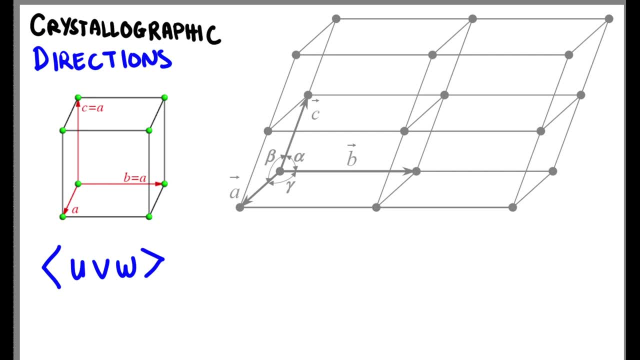 so take, for example, uh, in our cubic system. so the family of directions, the concept, this usually arises in your cubic systems. so we have, let's say, the one zero, zero direction. the one zero, zero direction here is ito, but in the cubic system this is crystallographically equivalent to: 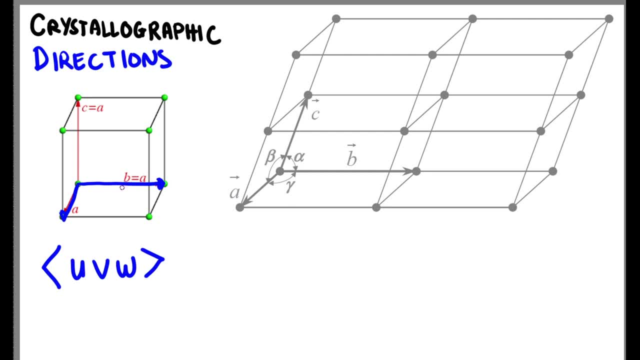 this direction here. this is the zero one zero direction and it's equivalent to this direction. this is the zero, zero one direction. so we can lump all these directions and yung kanilang reverse, yung paganyan, paganto and bababa, into one single family. so this will be the family of one zero, zero directions. 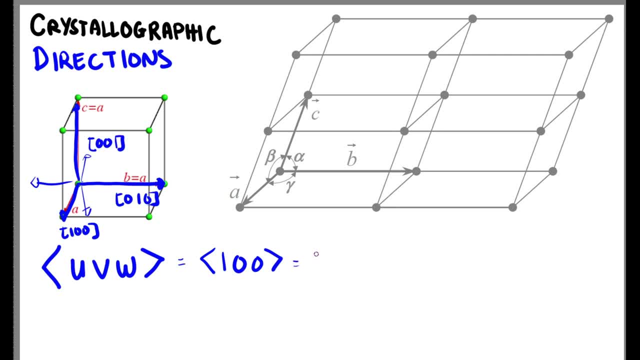 which is composed of the one zero zero direction, zero. one zero direction, the zero zero one. we have one bar zero, zero zero. one bar zero and zero zero, one bar. so do take note that the family of directions does not happen in all kinds of crystal systems. so hindi ibig sabihin na si one zero, zero, zero. one zero and zero zero one. 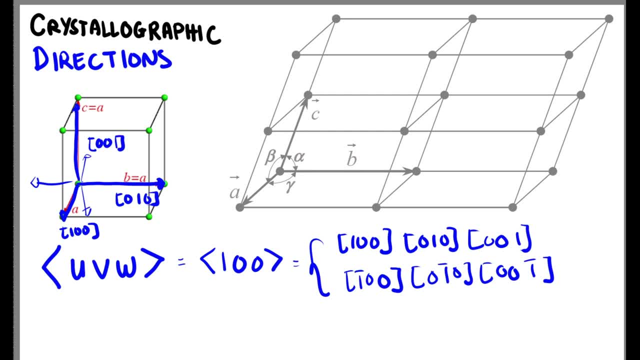 are crystallographically equivalent in your cubic system, that it will be the same as in, let's say, a triclinic system. so let's look back into our crystal. ito makita natin, yung one, zero, zero, ito, ito, yung zero, one, zero and zero, zero one. 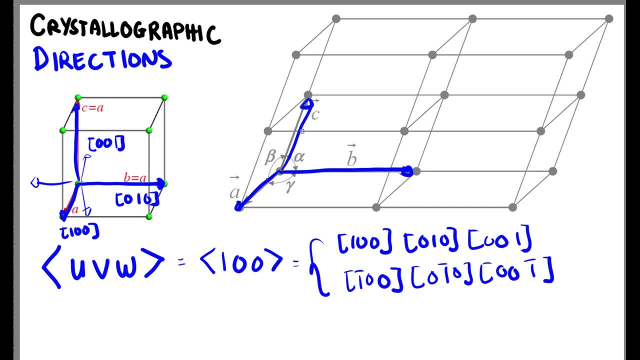 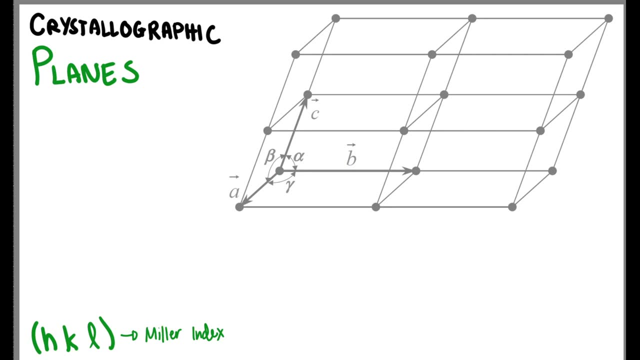 so makita natin yung lengths ni a, b and c are not the same. therefore they are not crystallographically equivalent. so this family hindi ito valid for this crystal system. now we go into our crystallographic planes. so the orientation of planes for a crystal structure. 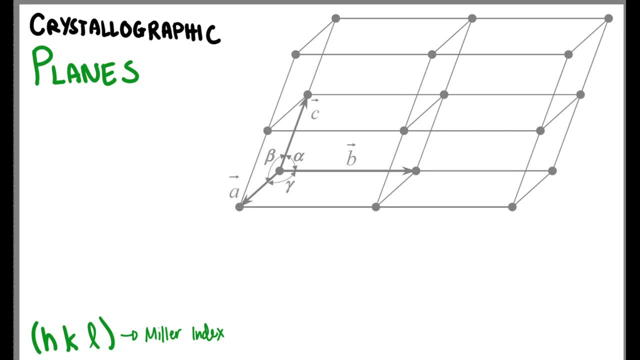 are represented in a similar manner, such as in our crystallographic directions. again, we use our three axis coordinate system with our unit cell as the basis of our like indices. so the crystallographic planes are represented by what we call the miller index, which has three indices: in the middle and the 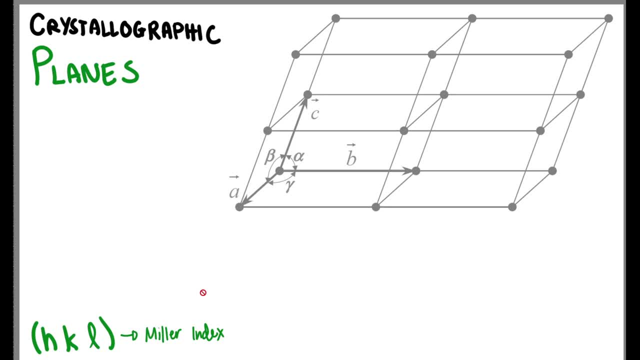 hkl. so this is for most crystallographic systems, and any two planes parallel to each other are equivalent and have identical indices. so the procedure to determine the hkl and index indices in the miller index system are as follows: first we ensure that the plane that we are concerned with does not hit the origin. 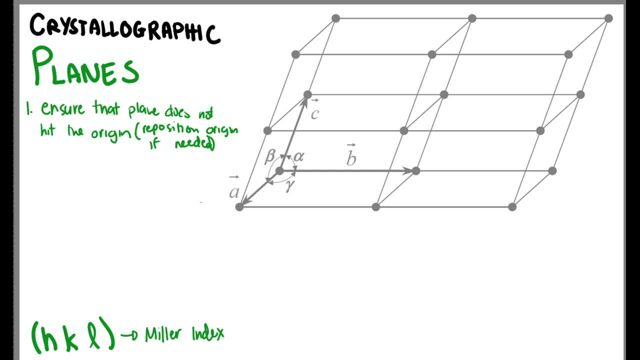 if it does hit the origin, we reposition the origin to another lattice point. in this case we do not comment on it. weikk 後. we take the intercept of the plane with all a, b and c and the intercept is measured with respect to our given origin or the new origin, if moved. 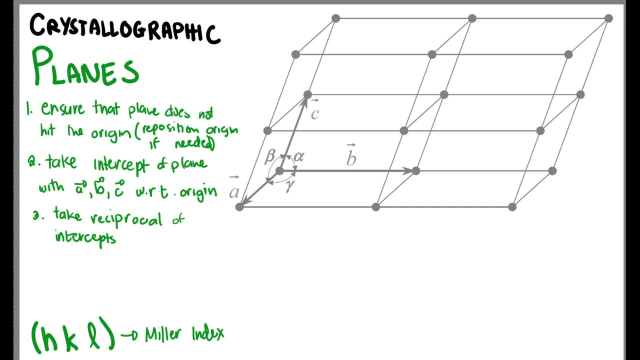 X kilonewa, then we take reciprocal of the intercepts, then, after which, if necessary, the indices are changed to smallest integral values. narras ontатель: In some representations we don't do this, but we'll cross that bridge when we get there. 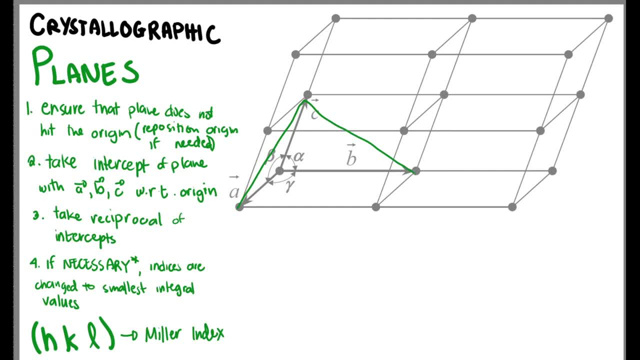 So, as an example, let's try this plane. So let's say this plane is plane P. So first step: we ensure that the plane does not hit the origin. So it does not hit the origin, there no need to reposition the origin. 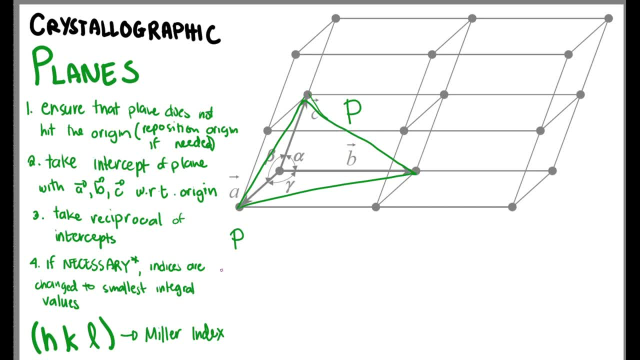 And secondly, we take the intercept of the plane with A, B and C. So here point P intersects A at 1, A intersects at 1, B intersects at 1, C. So we have 1, 1, 1.. 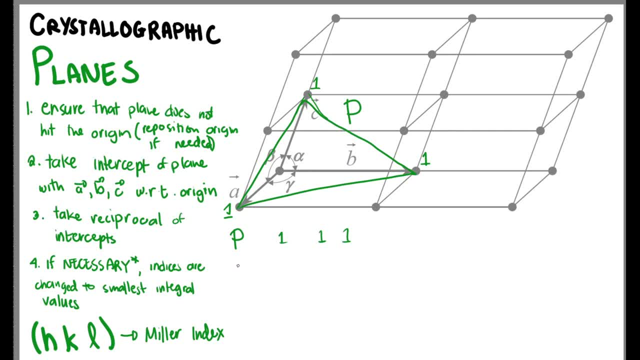 We take the reciprocal of the intercepts, and the reciprocal will be the values of H, A and L, where A is the reciprocal of this one, this one, this one respectively. So the reciprocal of 1 is 1.. So we have 1, 1, 1.. 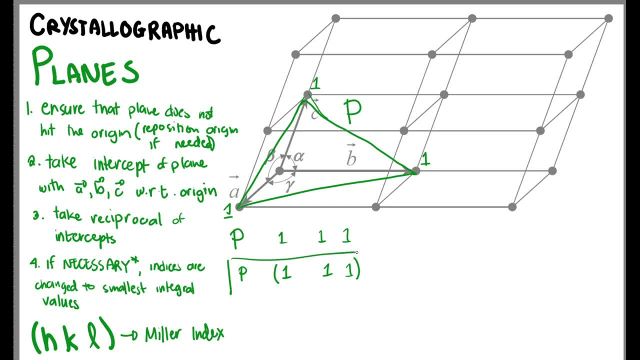 Then we enclose this in our parentheses and this would be the Miller index of this plane: P. So let's try a different example Now. let's try determining the Miller index of this plane. here This plane is P, So we followed these steps again to get the Miller index. 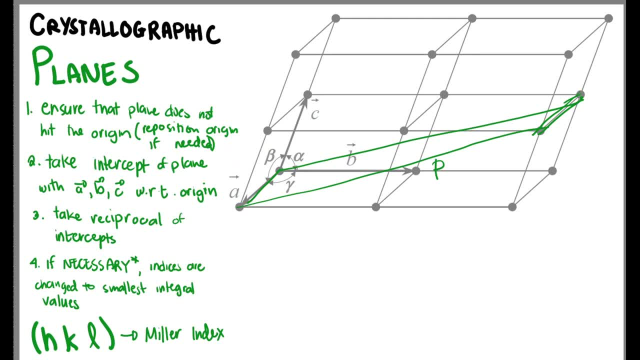 So first we ensure that the plane does not hit the origin, Since here it does hit the origin, so we can reposition our origin to another lattice point. So in my case, to make it simple, I'll just reposition the origin from here to here. 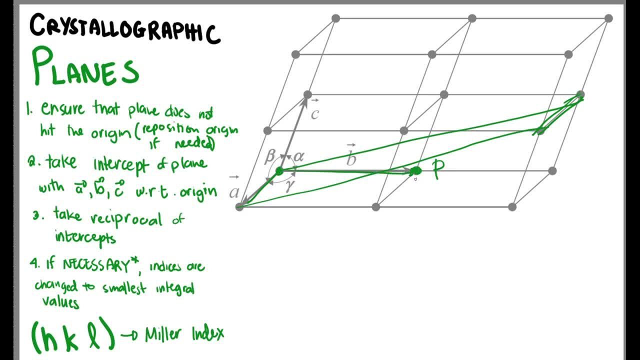 So this is our new origin. Okay, So let's make the origin. And here now we get to get the intercept of planes with A, B, C with respect to our origin. So our new A, B and C are here. 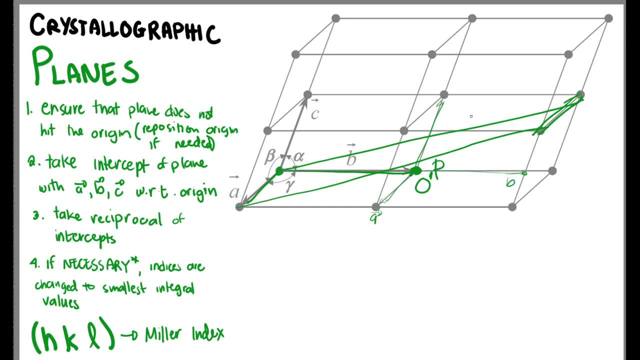 So this is A, B and C. So the intercept of this plane with respect to A. you can see it does not intersect A, So its intercept will be infinity. so this is for plane Q, infinity, the one with A. 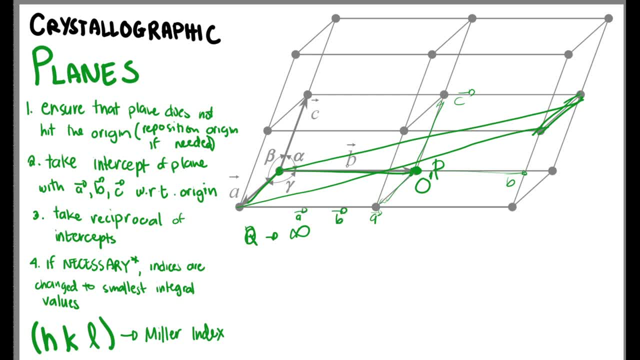 For B, its intercept is here: Here, If this is our origin and this is positive B, this will be negative 1B. And for C, its intercept is above: It is halfway down. Okay, Okay, Let's get through this one. 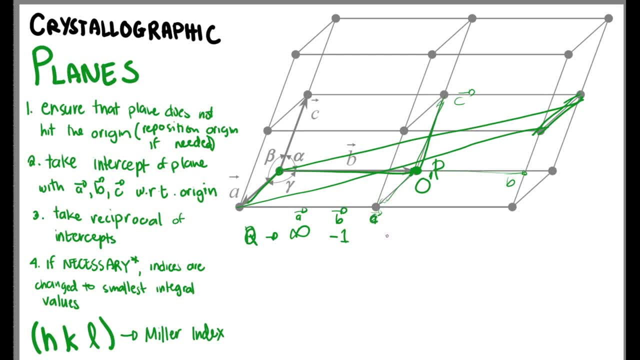 So we can say this is 1 half. Now we take the reciprocal of these intercepts, So to get the reciprocal reciprocal of infinity, so parallel to our axis is parallel to plane, Just take this in the meter index as 0. 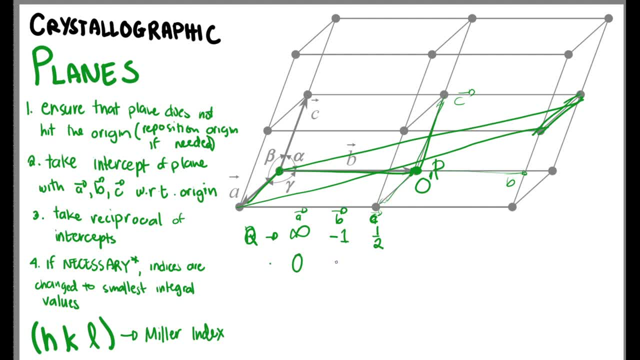 4B: reciprocal of negative 2.. 1 is negative 1 and for C the reciprocal of 1 half is 2.. Since this one is negative, we then change this to 1 bar, So we'll have 0, 1 bar 2. And no need to. 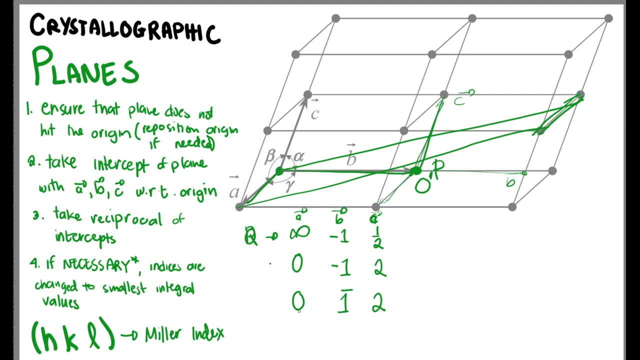 change the smallest integral value. since this is already the smallest integral value possible, We enclose this in our parentheses. and this is the Miller index for plane Q. Now let's say we want to create a plane given a Miller index. Let's say we get 1, 0, 1.. Miller index of 1, 0, 1.. How will we construct the plane? 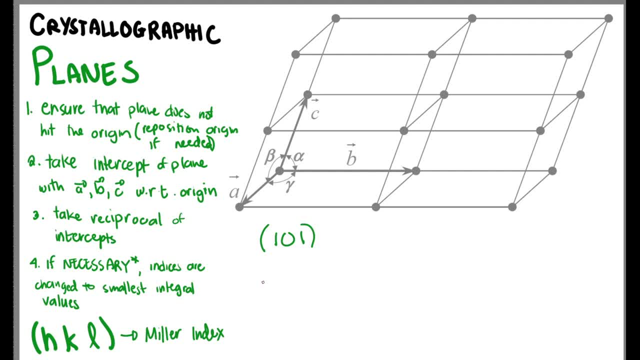 Basically, we just reverse what we did a while ago, So 1, 0, 1.. This means that the reciprocal of 1 half is negative 1 and the reciprocal of 1 half is 2.. Now let's say we want to create a plane given a Miller index. Let's say we get 1, 0, 1.. This 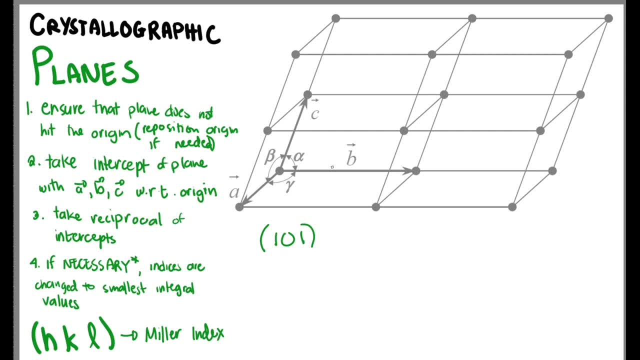 means that the reciprocal of 1 half is 2.. Now let's say we get 1,, 0,, 1.. This will be the intercept of the plane with respect to our origin. So getting the intercepts of each. we have intercept of 1, intercept of 0 is infinity. This will mean that the plane 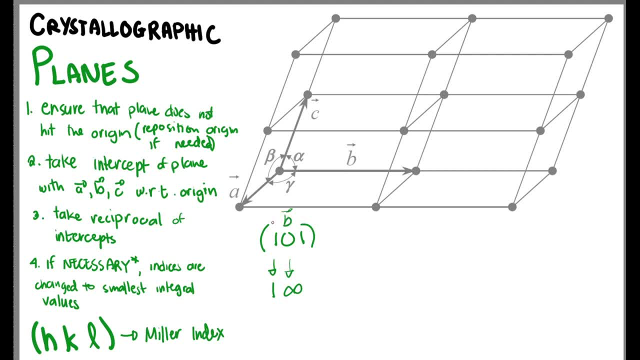 is parallel to the D-axis, And for C intercept of 1 is just 1.. So we just plot these points in our A, B, C here. So A it hits 1.. For B, it's infinity, So it hits 1.. And for C? 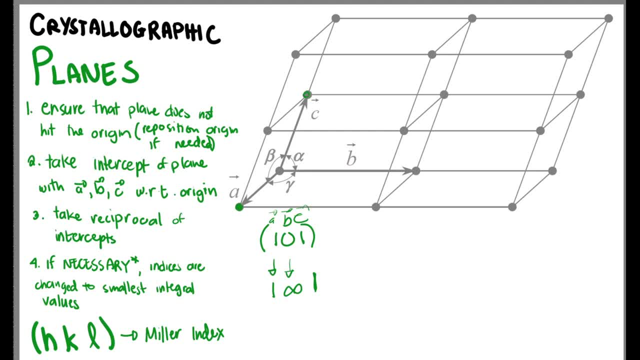 it does not hit the B-axis And for C it's the 1 there. So, tracing the plane, we get this plane. So, since it's parallel to B, we know that we need to make a parallel plane to this B-axis here, And this will be our 1, 0, 1 plane. So an important thing to note. 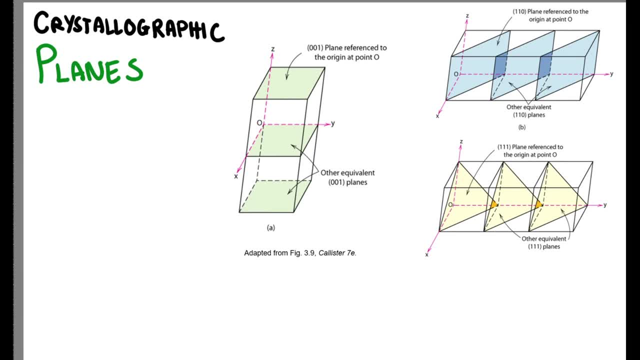 is that when we designate our planes in our unit cell or in our crystal- let's say we have a 1, 0, 0 plane or a 1, 1, 0 plane or a 1, 1, 1 plane- is that we're not only describing one plane, but we're describing 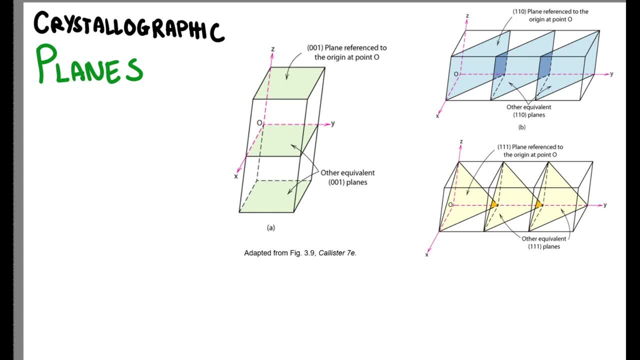 the connection of all of the planes that have that kind of orientation as seen here. So this is the 0, 0, 1 plane for this structure, This is the connection of the 1, 1, 0 planes and this is the connection of the 1, 1, 1 planes for this crystal structure. 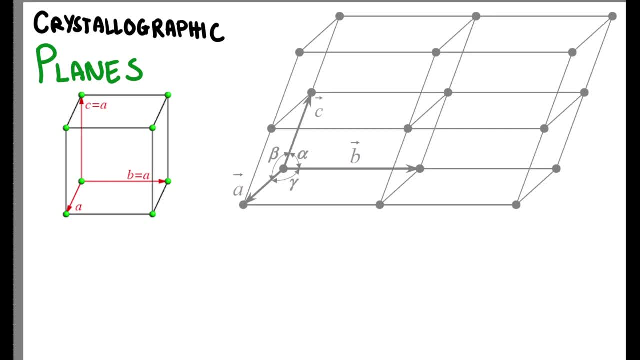 4. If in 0,, 0,, 0, 1 In crystallographic directions we have the family of directions, for some crystal structures, In the crystallographic planes we also have a similar concept called the family of planes. 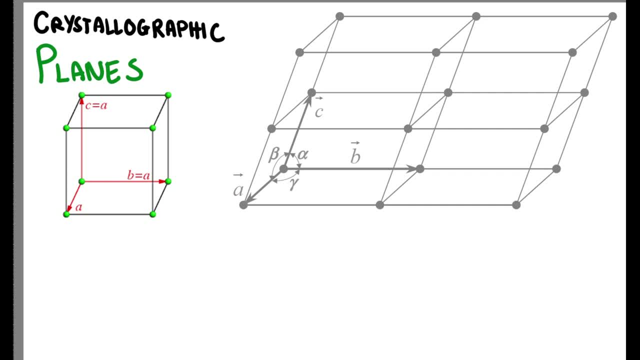 So a family of planes is just a set of planes that are crystallographically equivalent, So that is, they have the same atomic packing. So a family is designated by indices, kind of similar to our Miller Index, but instead of having, let's say, our plane is 111,. 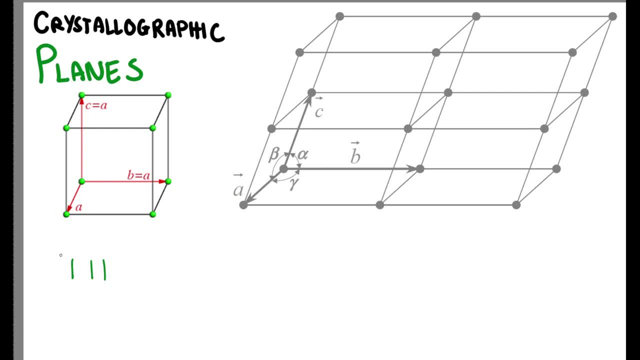 but instead of having a parenthesis, it's enclosed in curly brackets. So if our notation is like that, this is a family of planes. So let's see In the cubic structure this plane, this is our 001 plane. This is crystallographically equivalent to this one.